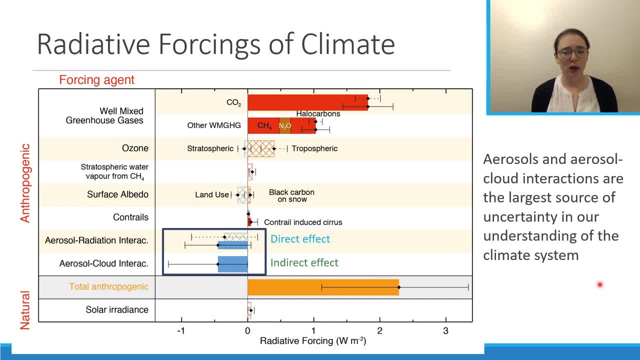 these error bars. aerosols and aerosol cloud interactions are actually the largest source of uncertainty in our climate system. Now, if you learned anything from module 5, which I hope you did, but I hope that you took away that aerosols are actually really complicated and measuring them- 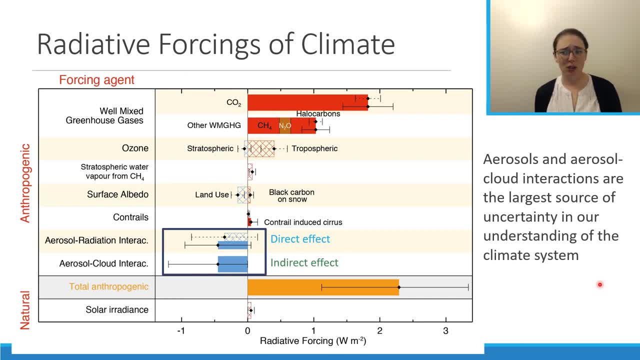 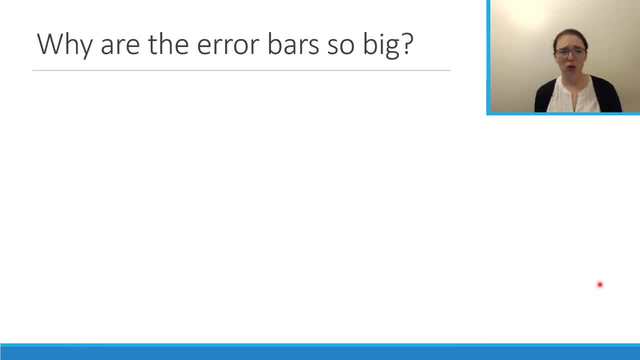 is hard. So that's one of the reasons the uncertainty is so great is actually there's just a lot of things about aerosols that we don't know. But the two major reasons those error bars are so huge is because our current climate models don't have high enough resolution to actually 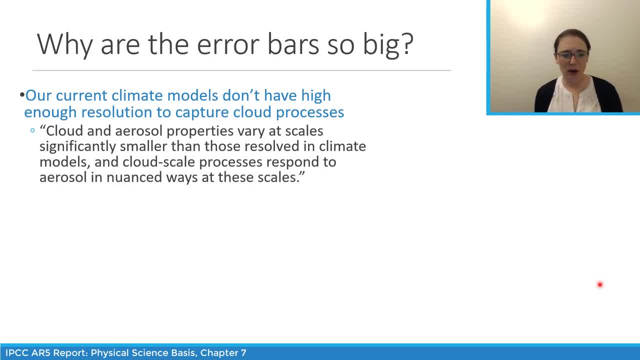 capture cloud processes. So I'll just read you a quote. Cloud and aerosol properties vary at scale significantly smaller than those resolved in climate models, and cloud scale processes respond to aerosols in nuanced ways at these scales. So when aerosols and aerosols are, 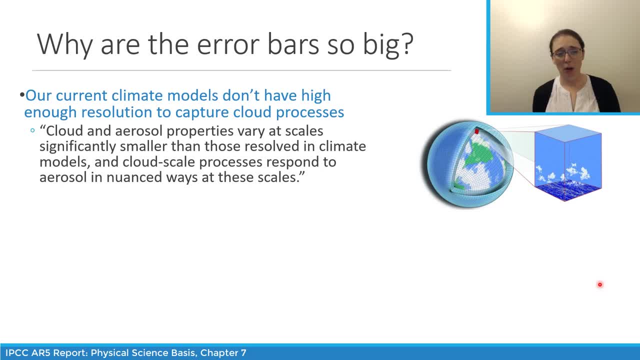 used in climate models. you have to split the atmosphere and the Earth's surface up into these grid boxes that essentially capture a little piece of the atmosphere and the Earth's surface, And then there will be essentially differential equations that will be solved for each of. 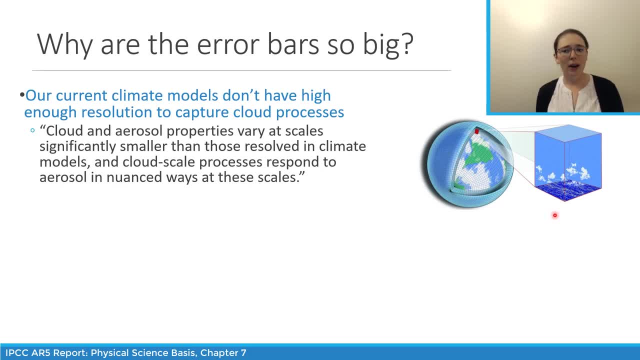 these boxes based on different parameters. Now for a global climate model, we're trying to do things like predict out to 2100 what the climate will look like, And so we're also trying to do that over the entire globe, and usually these atmosphere models are: 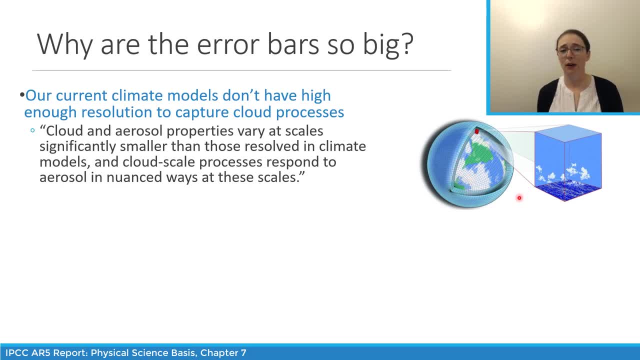 coupled to the ocean, So they're really really huge models that are very intensive to run, So these grid boxes have to be pretty big. Now, if I was going to run a local meteorological model for maybe the next two weeks out, I would probably use a much finer grid scale. but you just can't. 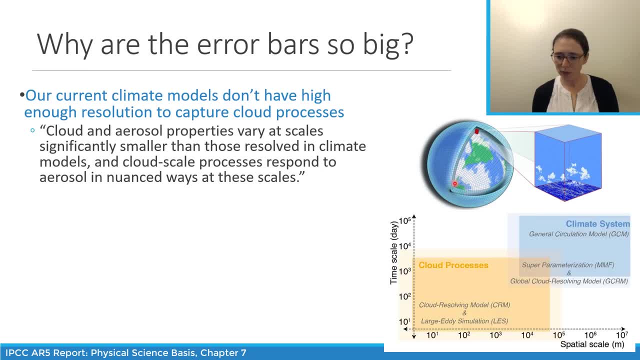 do that when you're trying to do this on the scale of a global climate model. So this is really one of the things that makes this error bar so big is that the models we use for resolving cloud processes are done on short time scales and small spatial scales, But for a global climate model. 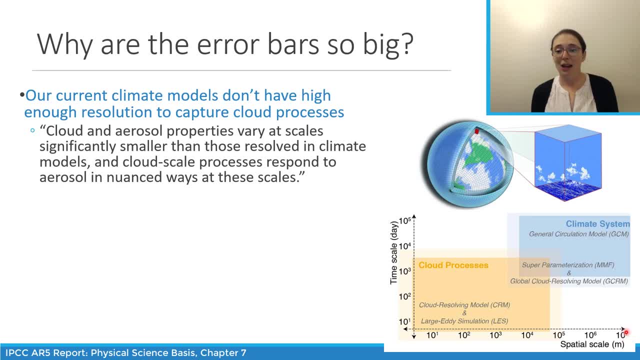 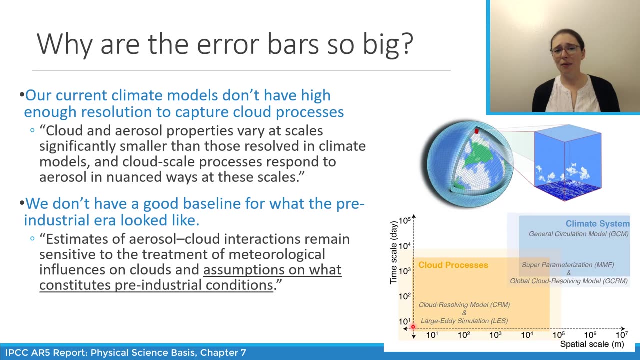 we're doing really big spatial scales- like the entire planet coupled together- and we're doing them over really long time scales like decades. So that's one reason that these cloud processes are really poorly resolved by the models. The second reason is that we don't have a good 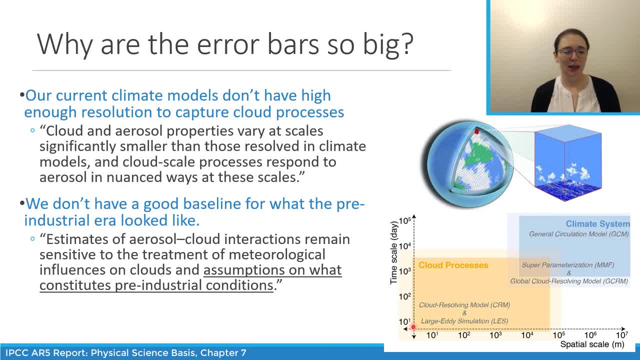 baseline. We don't know what that zero point really looks like in the pre-industrial era, So I'll read another quote. Estimates of aerosol cloud interactions remain sensitive to the treatment of meteorological influences on clouds and assumptions on what constitutes pre-industrial conditions. 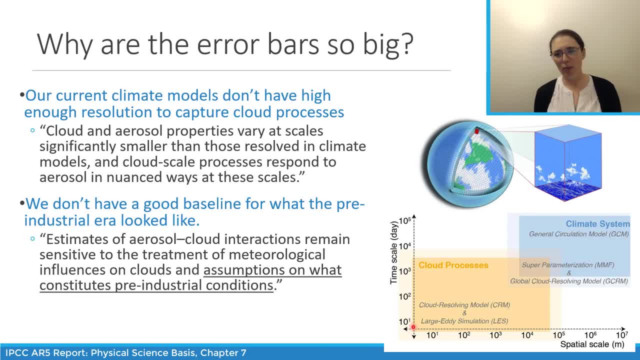 Now for something like carbon dioxide. we're able to actually get a pretty good record going back of what the carbon dioxide concentrations were thousands of years ago using ice cores. So basically, little bubbles get trapped in the ice core and you're able. 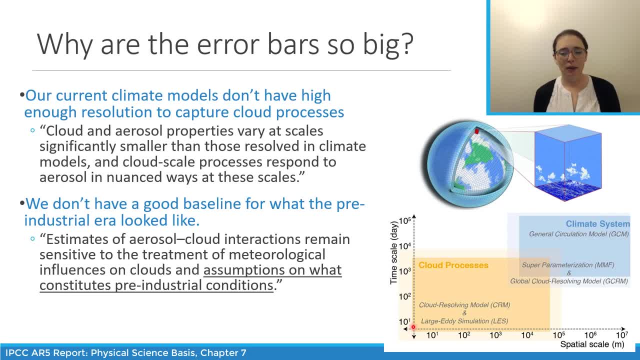 to measure the composition of the gas in that bubble and there's ways that they date how far back that layer of the ice core goes. You can do something kind of similar for aerosols, where you look for aerosols that have been deposited but aerosols aren't as well mixed. 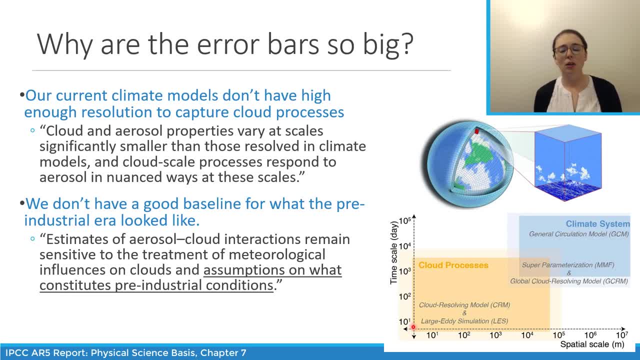 as carbon dioxide. So really you're only going to find the aerosols that are around over where you're taking your ice core from. So like they get a lot of them from Greenland, So you'll only know the aerosols that were deposited over Greenland and that doesn't tell you anything. 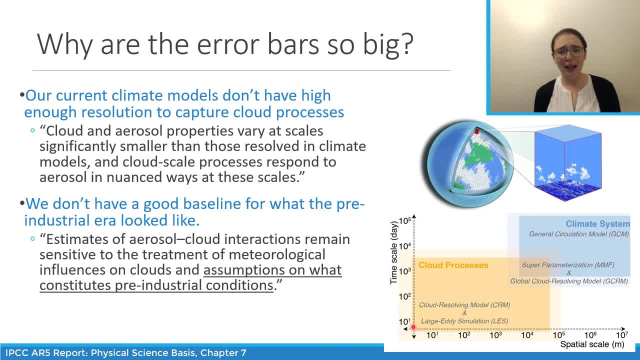 about cloud processes. There's really no way to get at what cloud coverage in cloud microphysics looks like before the satellite record starting in the 70s and 80s, So we really don't have a good pre-industrial baseline to compare our current day measurements to. 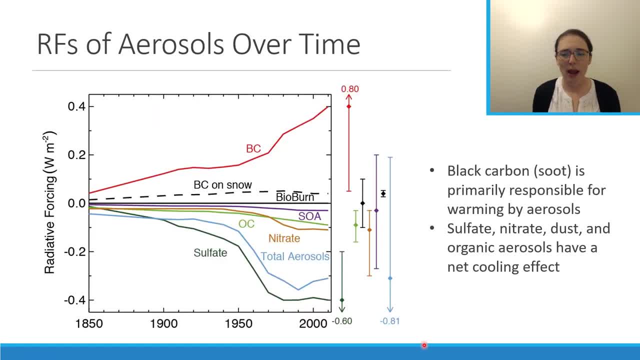 All right. so let's talk about the radiative forcings of different aerosol components over time. This is for the direct effect. so these are aerosol radiation interactions. So you can see our positive radiative forcing. So black carbon is primarily responsible for the warming by aerosols. 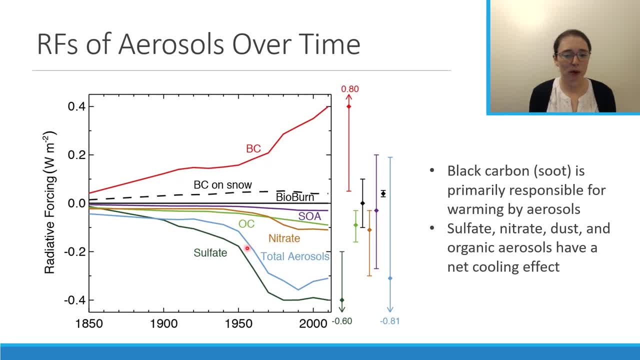 It absorbs solar radiation. And then our other components have negative radiative forcings, So these have net cooling effects. That includes our sulfate nitrate, organic carbon and secondary organic aerosol. And when we sum all these things up, 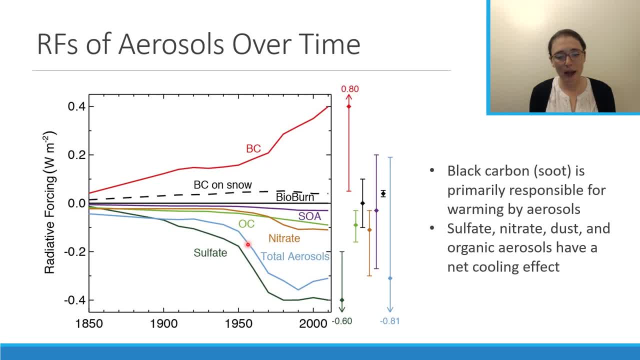 even since 1850, we've had a net cooling effect from aerosols. Now, you'll notice this only goes up to 1850.. The estimates from before that are pretty uncertain. There's really large error associated with them And you'll notice these things don't actually start at zero. That's. 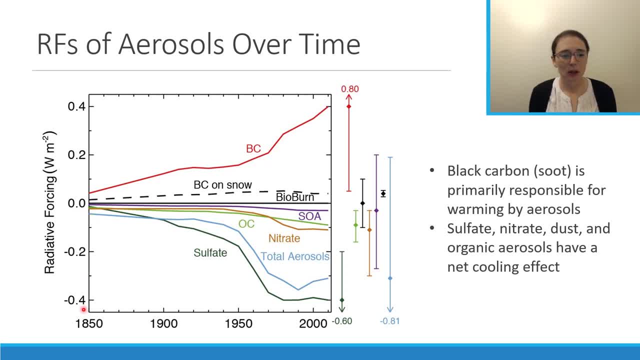 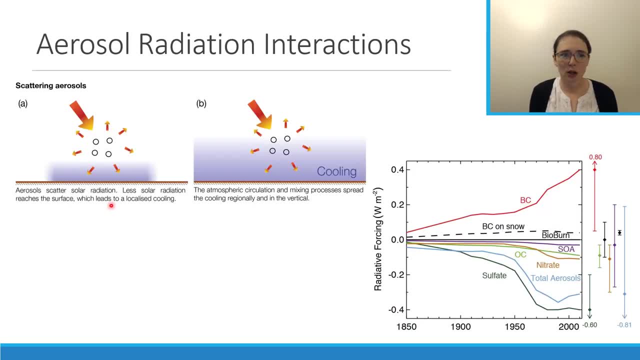 because there were aerosol perturbations before 1850, but we're pretty uncertain about where basically to put zero here. All right, so let's talk about some of these aerosol radiation interactions. So scattering by aerosols causes cooling, So basically light comes. 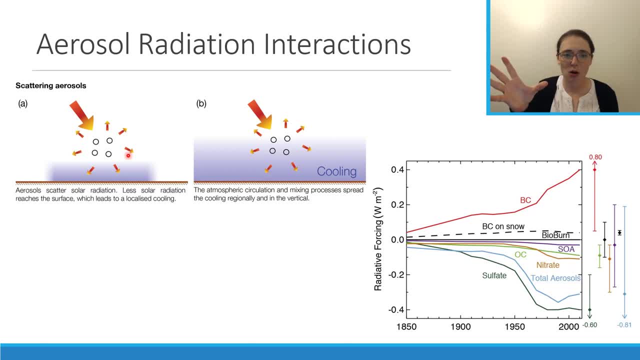 in and instead of continuing its downward trajectory, it gets scattered in all directions And you know about half of this light is going to be pointed upwards, about half pointed downwards or so. So scattering basically reduces the amount of solar radiation that reaches the Earth's. 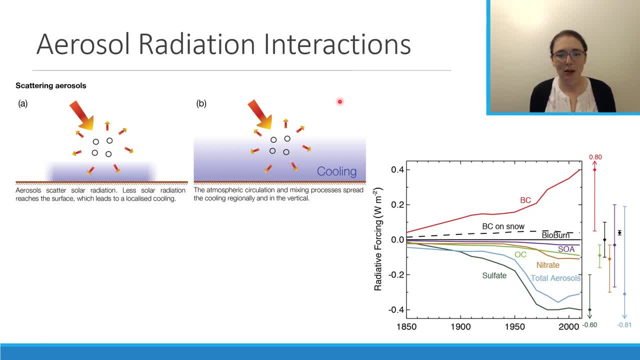 surface heats the surface less, So it has a net cooling effect. Now our absorbing aerosols is primarily going to be black carbon. I believe in another lecture we mentioned brown carbon as well, which just has some absorption effects. But basically the black carbon aerosols will absorb solar radiation. 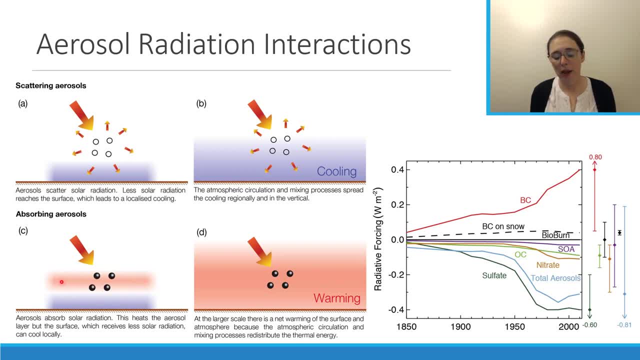 and this will heat the air in whatever layer these aerosols are in. Now most of our black carbon aerosol is going to be in the troposphere because, right, the lifetime of aerosols is pretty short, maybe two weeks, maybe a month at the most. That's not long enough to cross the tropopause. 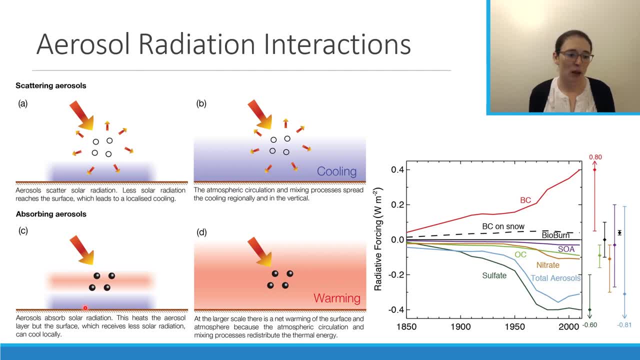 You're not going to get transport into other layers of the atmosphere. So the troposphere is well mixed. So even if you only have heating at the layer where this black carbon aerosol is hanging out, because of the general circulation in the atmosphere, 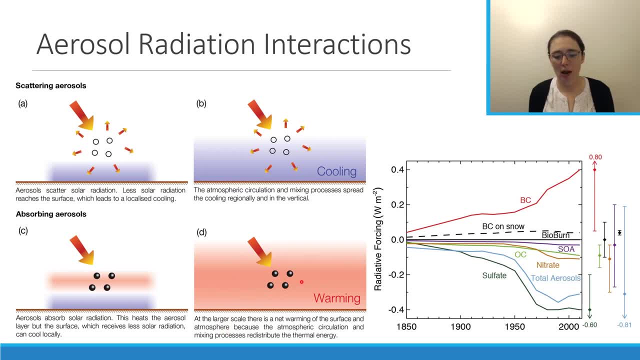 it will actually become well mixed and cause pretty much warming across the whole troposphere. Now I want to note something about this graph. Let's look at our sulfate trace real quick. So sulfate is scattering. obviously it has a negative radiative forcing. 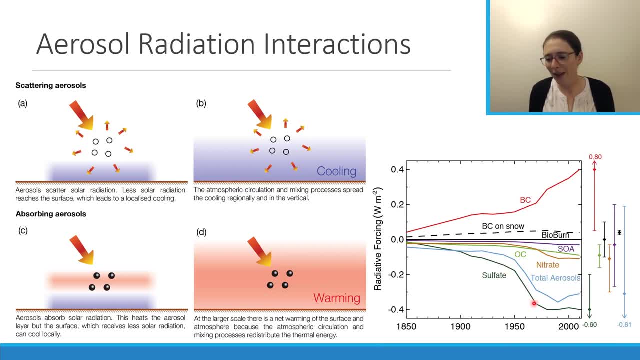 it cools. But let's look at sulfate, and sulfate looks like it actually levels out, starting about 1960, 70. Now what happened with sulfate in the 1970s? Let's think back to our lecture on acid rain. 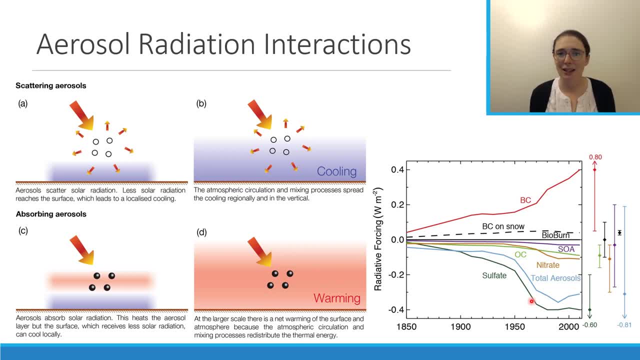 right. Acid rain became a really big concern in Europe and the United States and also some other countries, and they implemented a lot of SO2 emissions controls. So actually the sulfate-air-salt contribution has actually leveled off, But our black carbon has kept going up. So actually what we can see is our total. 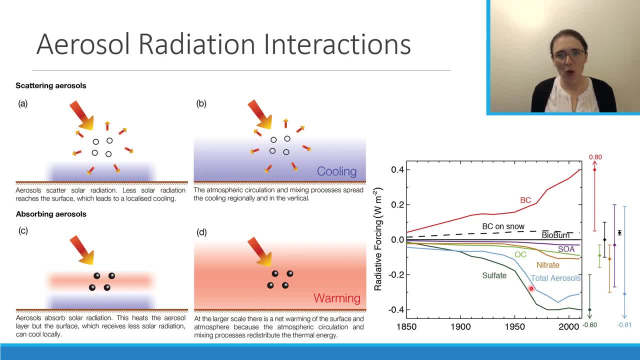 aerosol forcing. actually, over time it's still net cooling, obviously, but it's actually become a little bit less cooling because our sulfate, our biggest cooling influence, essentially has leveled off due to, essentially, sulfur dioxide emissions control based on acid. 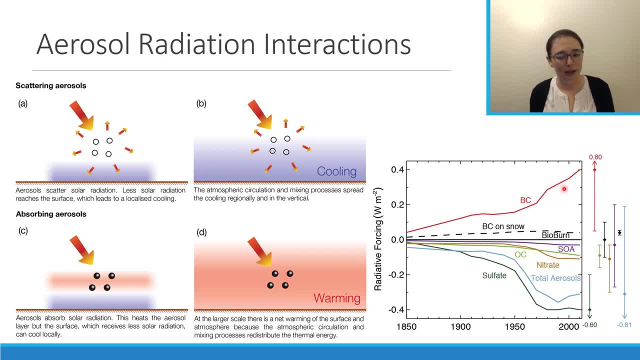 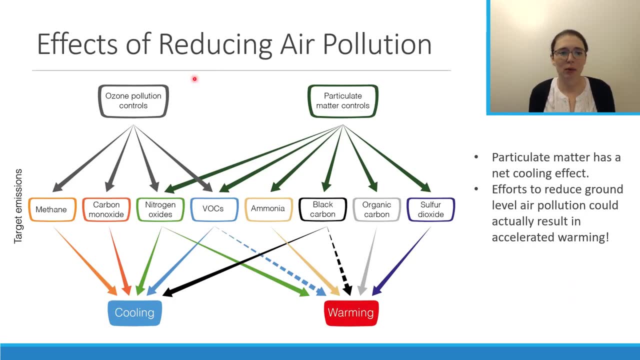 rain concerns and black carbon has continued to rise, So this doesn't bode well. So this leads into some of the effects of reducing air pollution. Now we talked about ozone during the greenhouse gas lecture. Ozone pollution controls reduce things like methane. 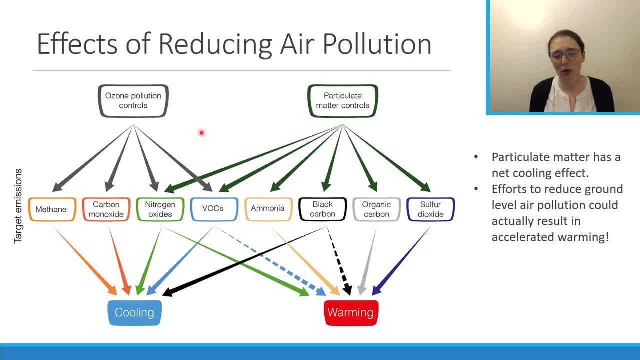 carbon monoxide, which are greenhouse gases. So actually reducing ozone- oh, and ozone itself is a greenhouse gas, So reducing the concentration of ground-level ozone actually has a net cooling effect. So this is good for climate change. but particulate matter controls actually remove things. 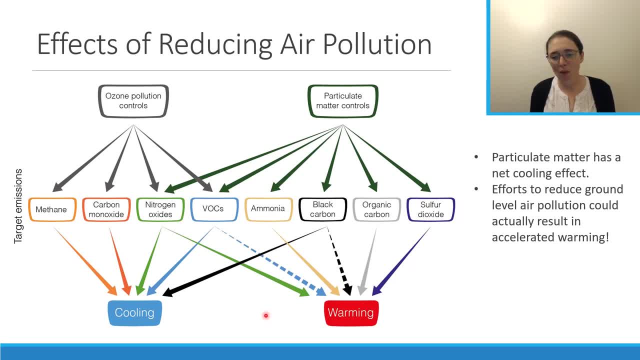 like organic carbon and VOCs, which form our aerosols, which scatter and reflect light. So actually, if you put in particulate matter controls, you could actually make global warming worse because you're taking away some of that negative radiative forcing that we have. 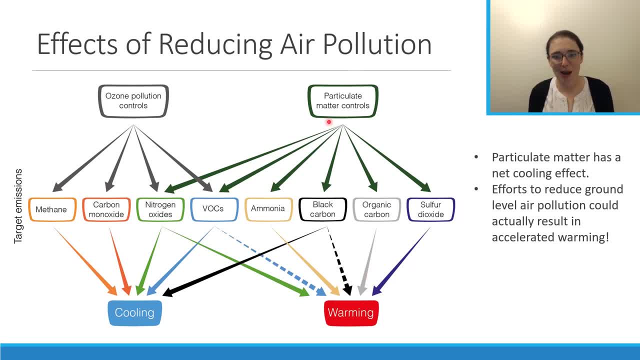 So this is not an argument for not reducing particulate matter. I mean, PM2.5 is linked to all of these horrible health effects, but it's just something that people need, that countries and governments need to consider when they're putting particulate matter. 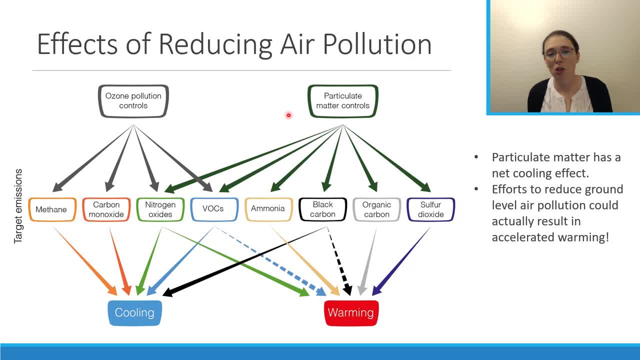 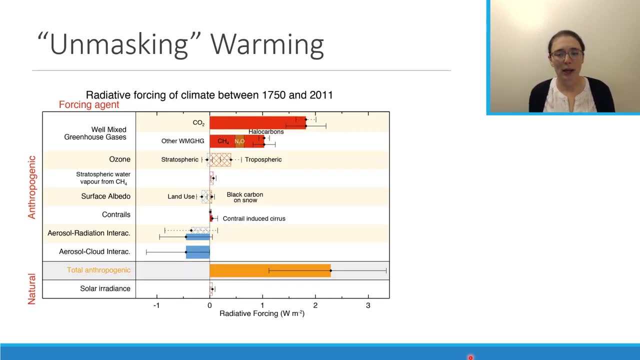 controls into place. Maybe you want to also put controls in for reducing CO2 or something to help offset the warming that will be caused by getting rid of particulate matter. So some people actually call this effect unmasking warming. So if we look at our aerosol effects, we see that they have a net cooling effect. 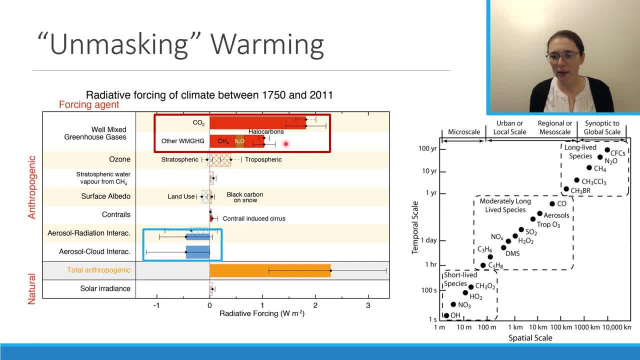 and our greenhouse gases all have a net warming effect. Now, this is a throwback to Module 2, when we talked about the lifetimes of different species, and something you'll notice are these greenhouse gases are all long-lived species. We have methane with a lifetime of a little over 10 years, nitrous oxide- even longer CFCs, you know. 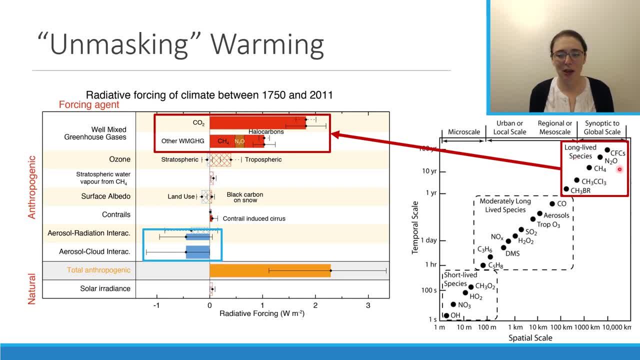 over a century. CO2 is not on this chart, but if it was, it'd be hanging out here. So these are going to stick around for a long time and they'll keep contributing to the radiative forcing of the Earth as long as they're in the atmosphere Now. 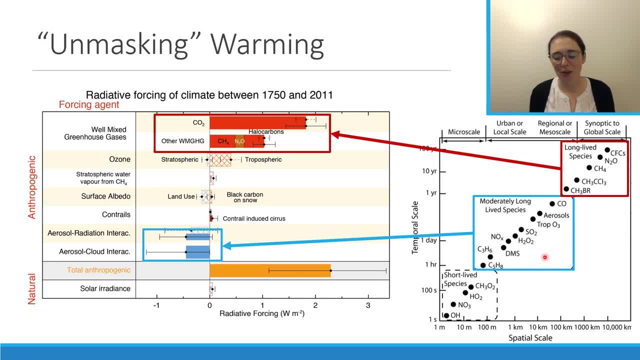 our aerosols have shorter lifetimes and also the aerosol precursors also tend to have short lifetimes. So aerosols, the right-sized aerosol, under the right conditions, can stay in the atmosphere for a couple of weeks at the most, maybe a month if it really gets lofted up high. but yeah, these lifetimes aren't that. 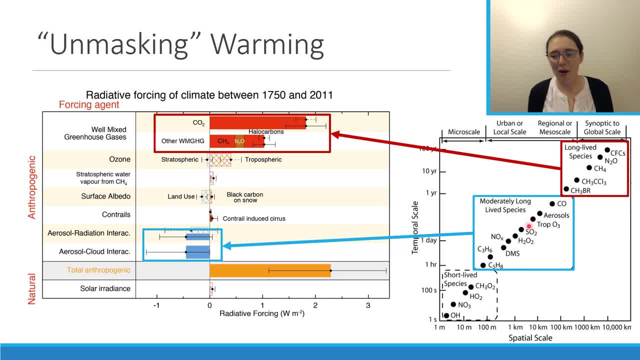 long for aerosols. So if we stopped emitting particulate matter and our aerosol precursors like SO2 tomorrow, we would actually see a big acceleration in the net warming effects of these greenhouse gases because we would unmask them, We would take away essentially this buffer on the system. So 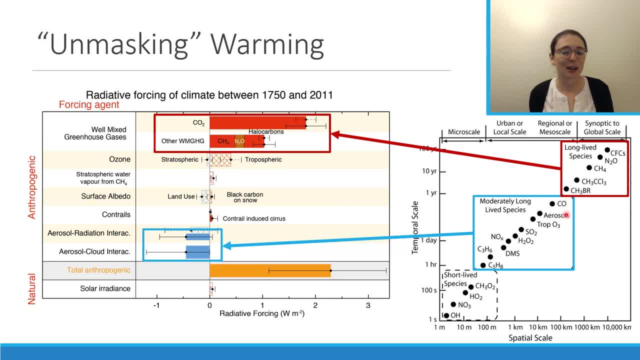 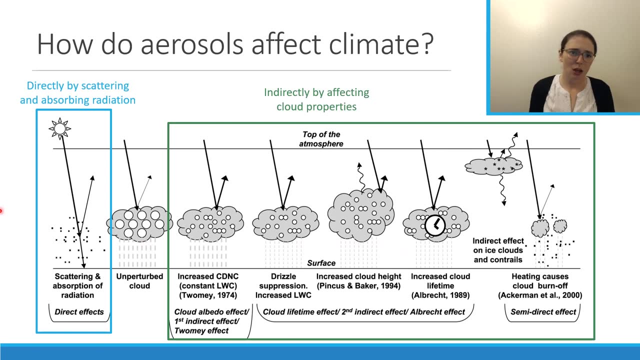 this is something that a lot of people are concerned about. as countries clean up their air pollution, which is really good for the people there, We also need to put greenhouse gas emissions control into place, otherwise we risk essentially accelerating climate change by unmasking the aerosol effect. Alright, so switching gears, so we've all we've. 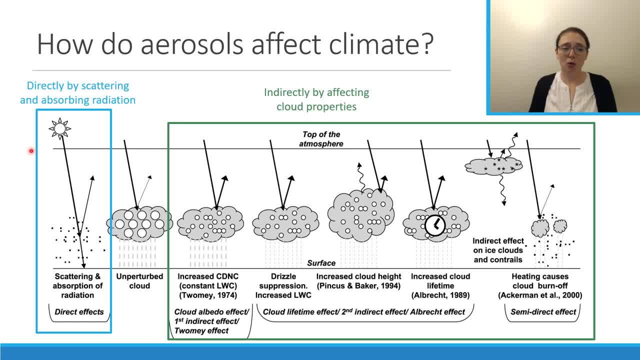 been talking about the direct effect so far, so scattering and absorbing by aerosols. Now I'm going to switch gears to talking about the indirect effect. so that is the effect on cloud properties. Now I'm not going to go through this diagram in detail, but look how. 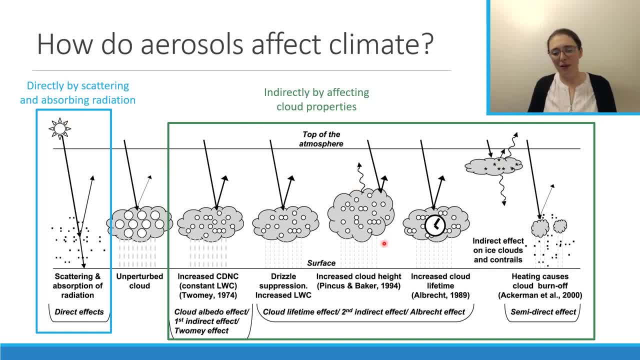 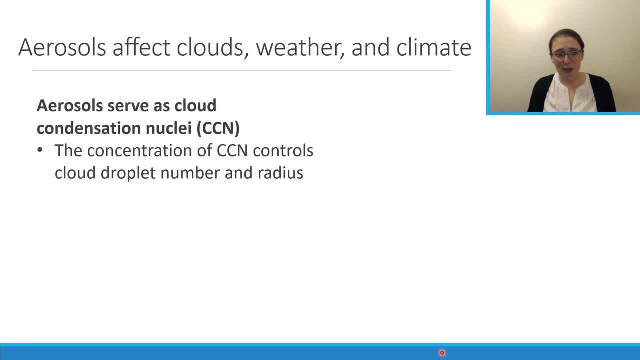 small this box is. Look how big this one is. All of these different effects, aerosol-cloud interactions are actually really complicated, So let's start with the basics. Aerosols serve as cloud condensation nuclei, So essentially that is a cloud seed, You have a particle and water vapor. 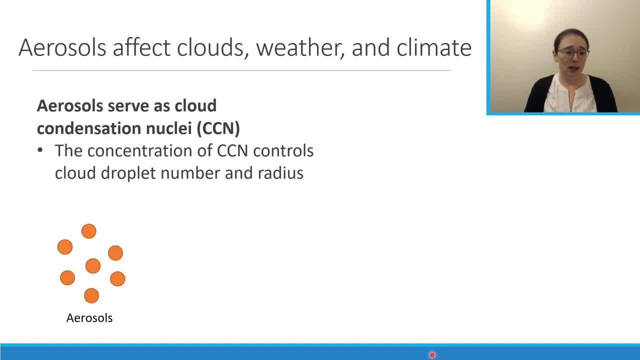 condenses onto it. So let's look at what that looks like. We have some aerosols in the atmosphere. Water vapor is going to condense onto them, forming droplets. this will form a cloud, and then the number of cloud condensation nuclei, the. 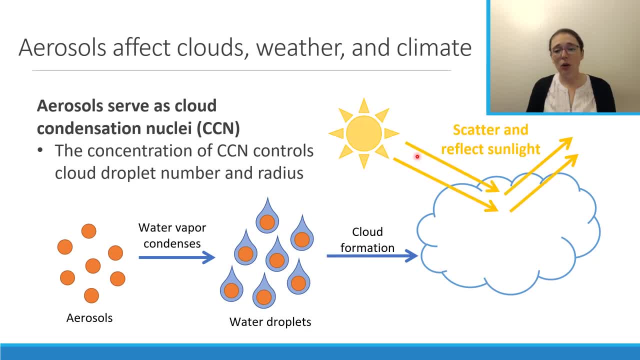 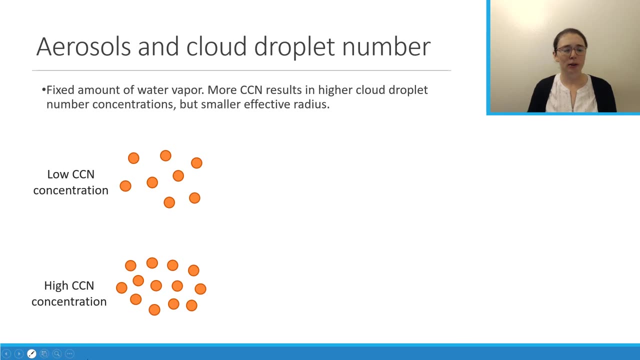 number of aerosol particles that can serve as cloud seeds is going to affect how that cloud scatters and reflects sunlight, so solar radiation. it's also going to have effects on precipitation in the cloud lifetime. so let's talk about how aerosols actually affect these cloud properties. so let's consider a 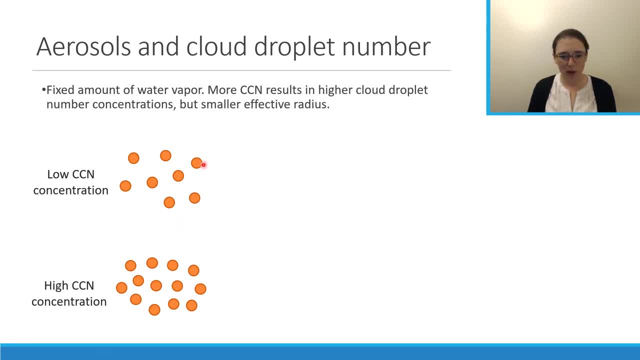 situation where we have a low CCN concentration, so not a lot of particles in the atmosphere. this would be probably more representative of a pristine condition in a lot of places. under these conditions we'll get a lower number of large droplets. so there's a fixed amount of water vapor in the air parcel and if 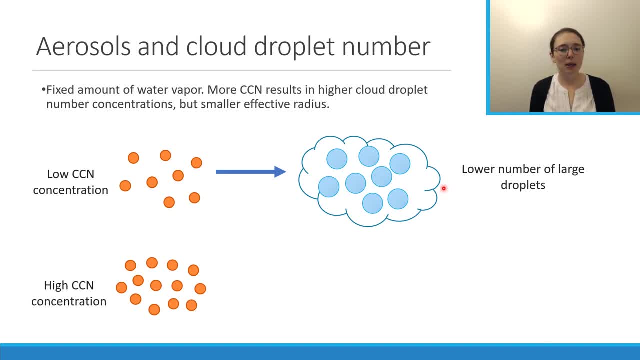 we have less seeds, we have more water vapor that can be basically condensed onto each of these seeds, so there's more water vapor to go around. so the droplets grow larger. so low CCN number, low droplet number, but then bigger droplets because there's more water vapor available now if we have a high. 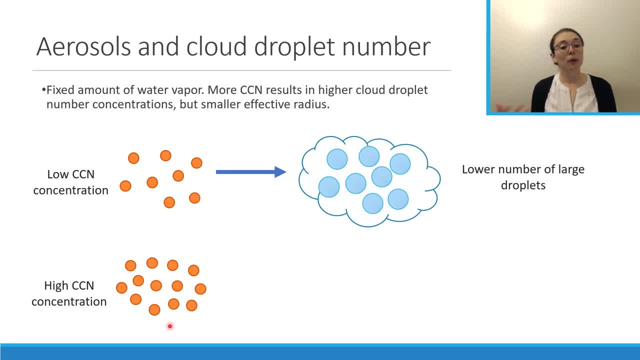 CCN concentration, for example, pollution outflow or lots of SO2 pollution that's causing nucleation of new particles, new sulfate particles. so if we have a high CCN concentration, well, we'll get a larger number of cloud droplets, but smaller because there's that same amount of water vapor to go around to each. 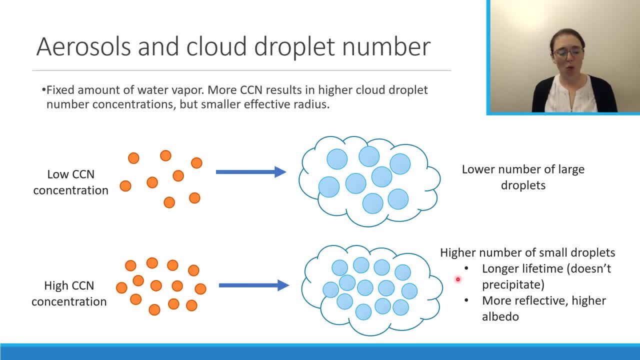 particle, but since there's more particles taking up water, each of these droplets will end up smaller. the basic result of this is that these clouds have a longer lifetime because, since the droplets are smaller, they don't precipitate as quickly. they might actually evaporate before they form. 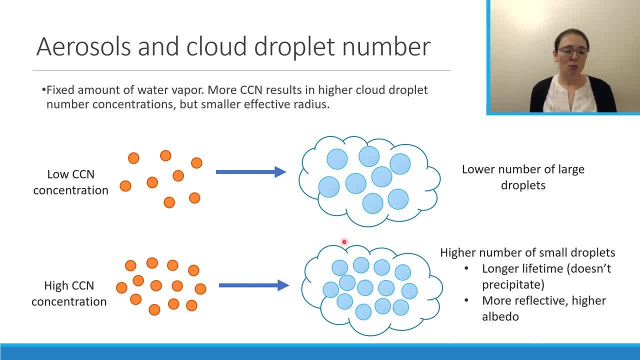 precipitation before they rain out. they're also more reflective because smaller droplets are brighter, they reflect sunlight better, so these clouds are actually more reflective and longer lived. so this is why aerosol cloud interactions actually results in a net cooling effect is because when we put particles into the air, we make these. 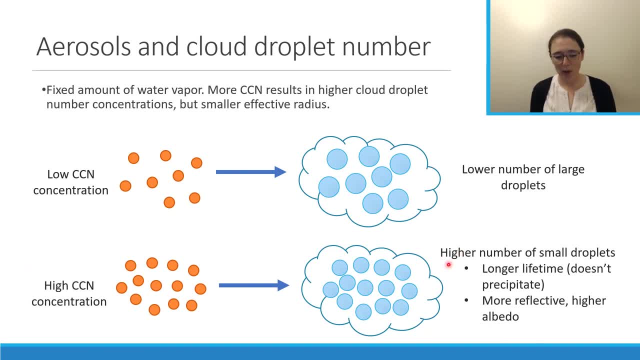 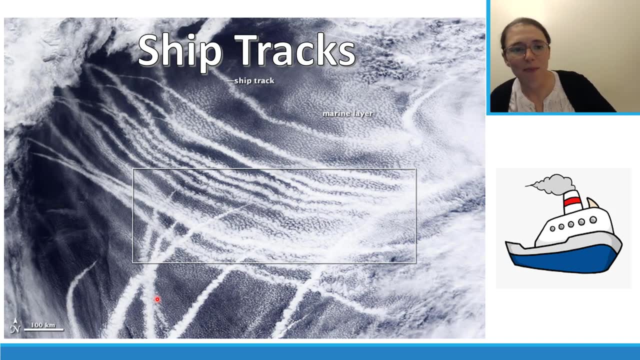 clouds more reflective and we give them longer lifetimes from our pollution, from our formation of anthropogenic aerosols, all right. so my favorite example of this is ship tracks. aerosols are real, cloud concentration nuclei are real and I can prove it to you with this picture. 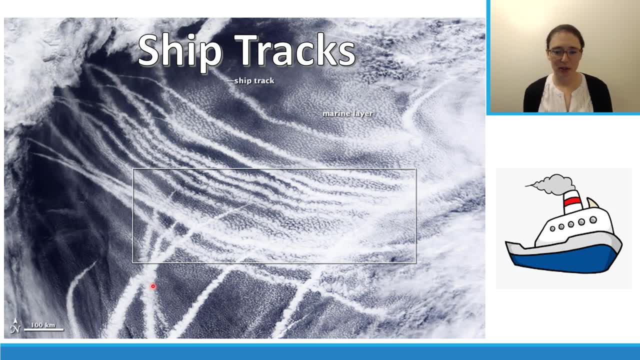 so this is a satellite image showing a shipping lanes. this is where big ocean going ships are going through, so we see our dark ocean in the background and then we have clouds now all around. we have kind of these pretty transparent light cloud cover. it's really not thick clouds, except in these tracks. this is 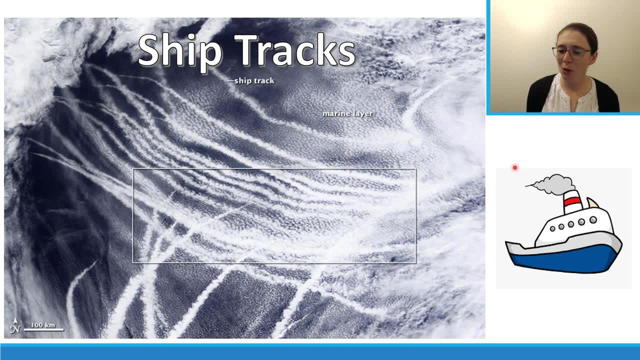 where a ship has gone through and the ship has been spewing particles from its smokestack. so we have a ship go through, it spews lots of particles and then you get the formation of these really bright cloud tracks. that tracks really exactly right where the ship went through. so these 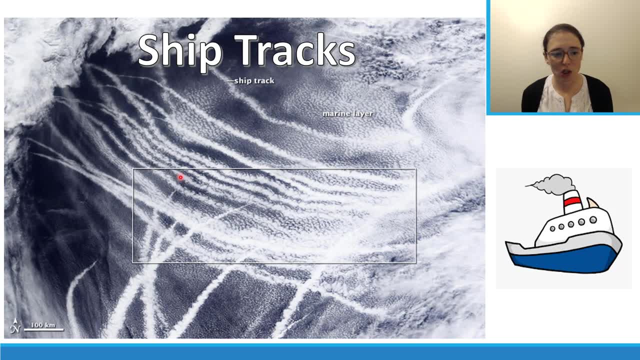 clouds are brighter, they're fluffier, they're reflecting more radiation. right, because the ocean surface is dark, the ocean service absorbs radiation. you know, you know this intuitively, right, if you're in a parking lot of summer day, the black car is gonna be warmer than the white car. 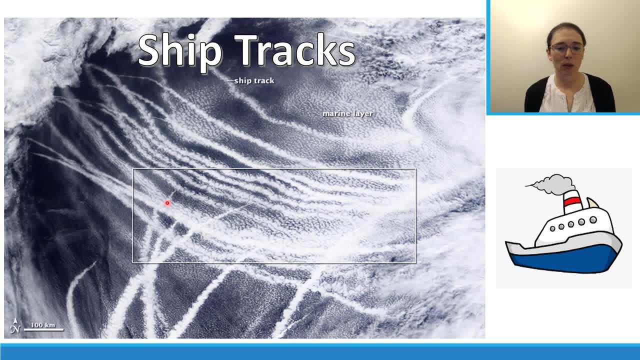 So the thick clouds are reflecting more light. Less is getting to the surface, And this is simply due to, essentially, an infusion of particles from a ship that has gone by. So I just think this picture is so cool that you can actually see so clearly the effect of particles. 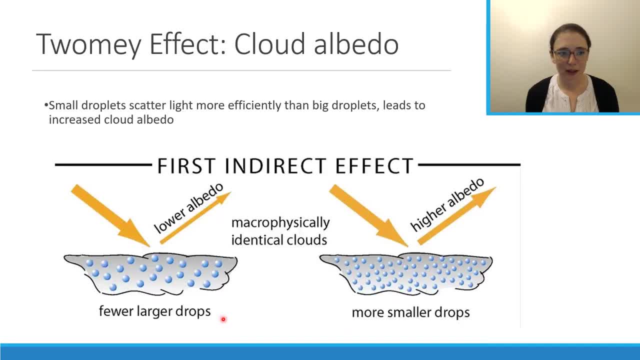 on clouds. So let's talk about the indirect effect. There's basically two major facets of the indirect effect. we talked about this before, But one's called the Tuomi effect. So this is how, basically, smaller droplets scatter light more efficiently than big droplets, which increases cloud albedo. 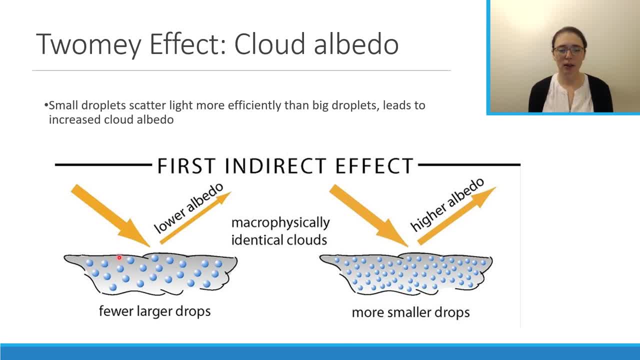 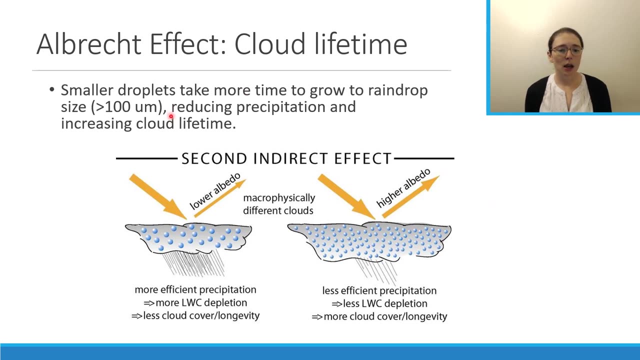 makes the cloud brighter. So we have a few large droplets, less reflection. But when we have more small droplets we get higher albedo, so more reflective clouds. The second indirect effect is the Albrecht effect, which is the effect on cloud lifetime. 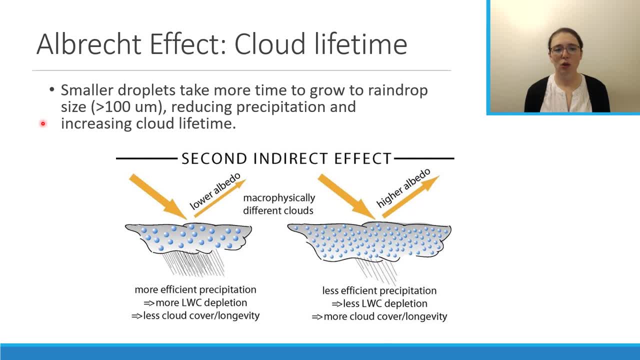 So basically smaller droplets. The second indirect effect is that smaller droplets take more time to grow to raindrop size, which reduces precipitation and increases the lifetime of the cloud. So if the cloud is going to stay around in the atmosphere longer, it's going to reflect more light over its lifetime. 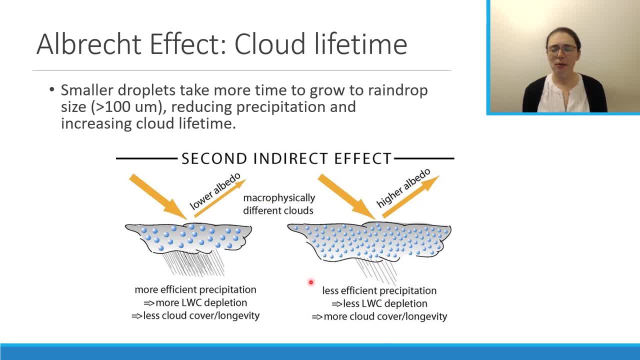 It also decreases precipitation, So this cloud has basically a higher likelihood of evaporating. before it actually precipitates, It rains out, which keeps water vapor in the atmosphere. So, yeah Yeah, Indirect effect is basically the effect on cloud lifetime. There's also a lot of other there's. 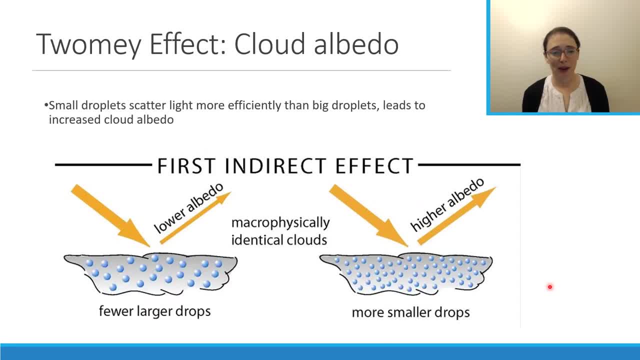 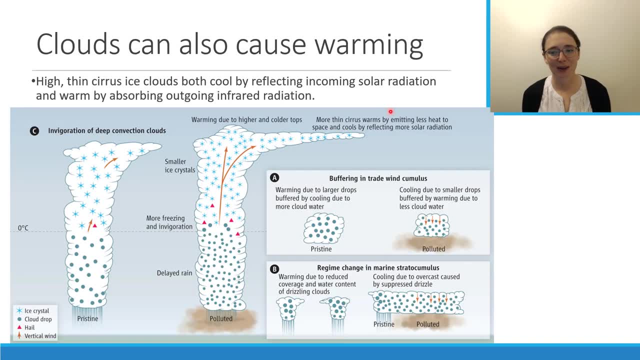 lots of effects aerosols can have on clouds. These two effects are our major ones, But, for example, clouds can also cause warming, right? Just because you needed one more thing to be confused about. So basically, very high, thin cirrus clouds. 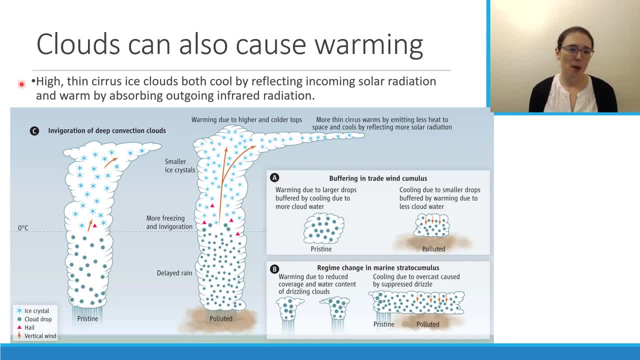 are going to freeze because it's really cold in the upper atmosphere. So these clouds are going to form ice crystals, So they'll be frozen. And that ice crystal, it can reflect incoming solar radiation, but it can also warm the atmosphere by absorbing infrared radiation. 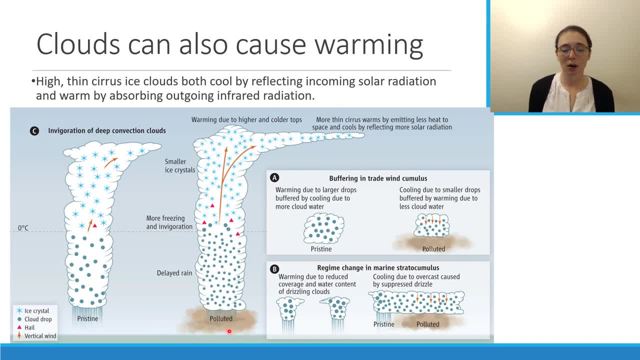 So there's some evidence that the increased CCN number under polluted conditions can actually cause clouds to rise higher in the atmosphere because they're not raining. They can continue to rise and then you can actually get more thin cirrus ice clouds that could cause warming. 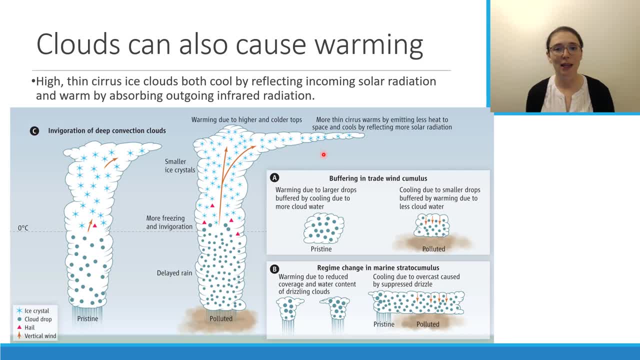 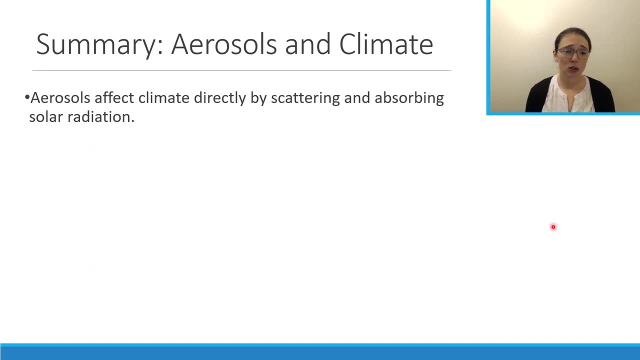 So, yes, there's a lot of different things that can happen with clouds and aerosols, But overall, aerosol- cloud interactions do have a net cooling effect. All right, that is the end of the lecture on aerosols and climate. So just to recap, we talked about how aerosols 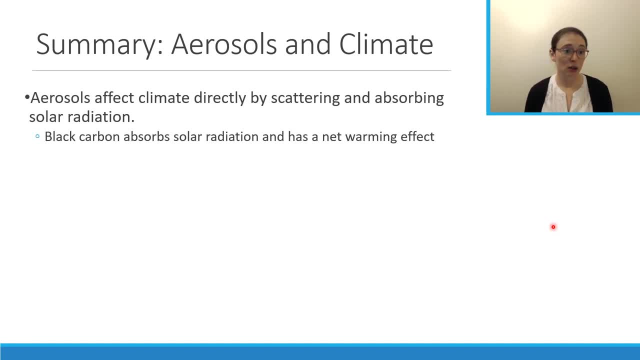 can affect climate directly by scattering and absorbing solar radiation. Um Black carbon absorbs solar radiation, has a net warming effect. Other aerosols like sulfate dust, organic carbon et cetera, scatter light and they have a net cooling effect. 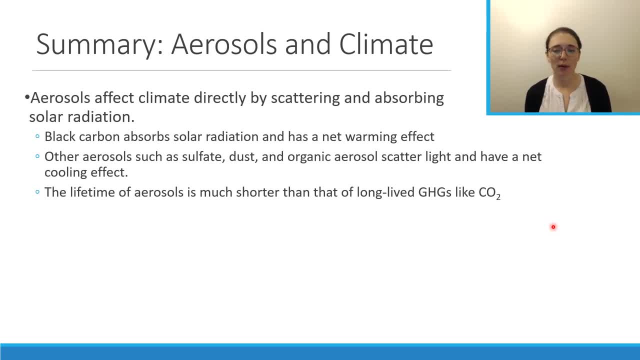 And we talked about how the lifetime of aerosols is so much shorter than that of a long loop greenhouse gas like CO2, which means that we essentially, if we stopped emitting particle pollution, we could accelerate warming by removing some of that negative radiative forcing from the aerosol. 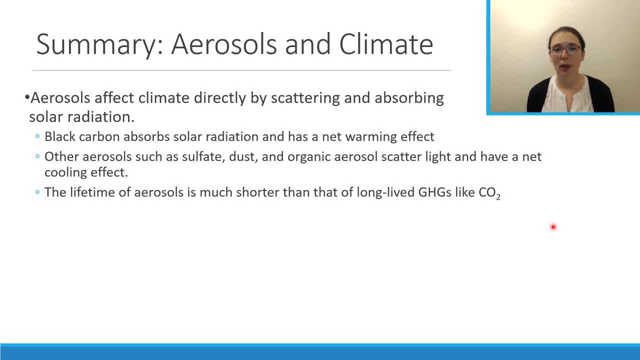 effects, While the lifetime of CO2 is so long that radiative forcing is in the atmosphere for a long time. All right, we also talked about how aerosols affect climate indirectly, by affecting cloud formation and properties. So aerosols serve as cloud condensation nuclei, or CCN.